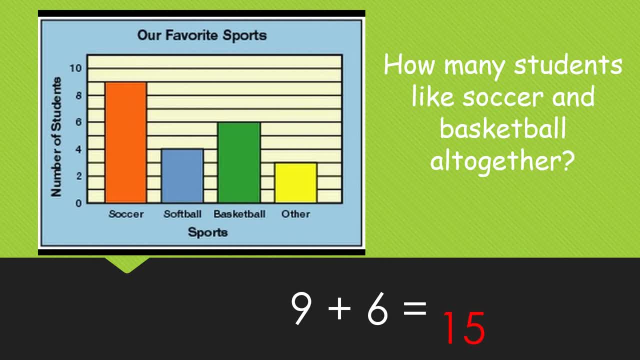 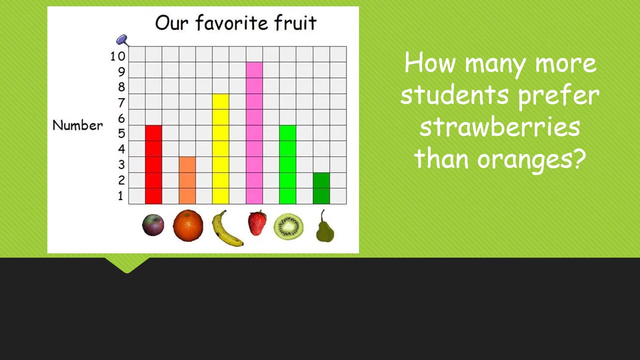 nine plus six and that equals 15.. Stand up and do 15 jumping jacks- Great job. Let's look at our favorite fruit. How many more students prefer strawberries than oranges? The way we figure this one out is whenever you hear how many more that is. 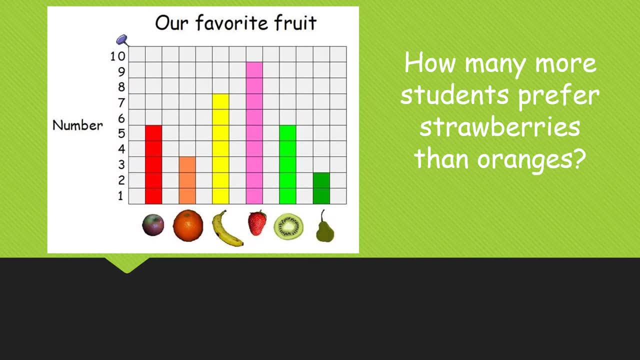 automatically a subtraction problem. How many more students prefer strawberries than oranges? We find this because strawberries have nine people who liked that, and then oranges have three. So nine minus three equals, yes, six. It is your turn to do six crab kicks. 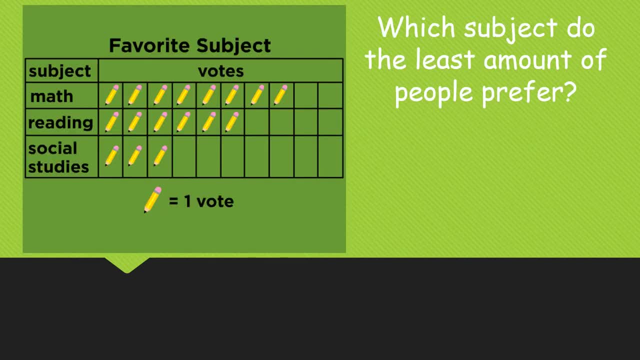 You're doing awesome. Keep it up. Next one: This is a graph, a pictograph on favorite subjects. Which subject do the least amount of people prefer? The least amount means the smallest amount- Yes, social studies. It only has three votes. Go ahead and do three lunges. 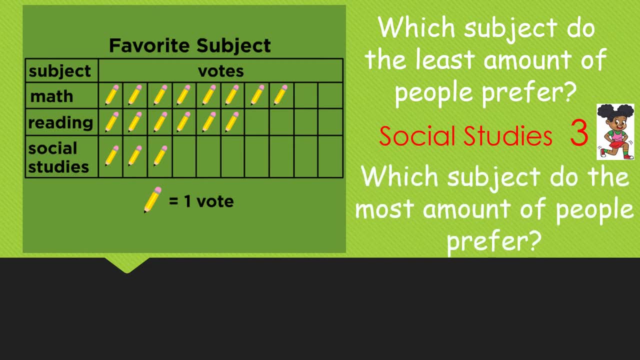 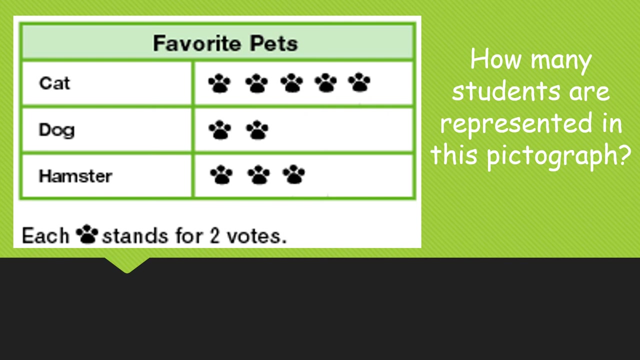 Awesome. Next one: Which subject do the most amount of people prefer? Yep, that is math, and math has eight people who prefer it. Great job, Go ahead and do eight windmills, All right. next one. Now let's look at this favorite pets pictograph. 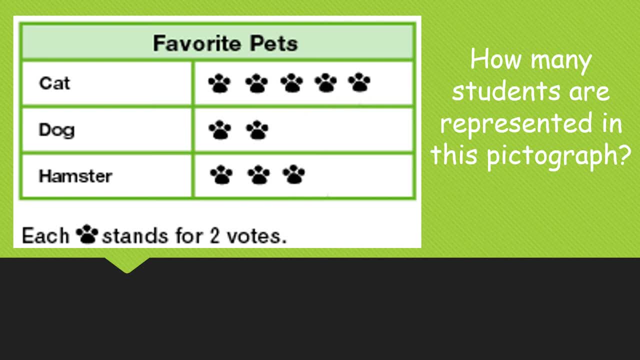 How many students are represented in this pictograph? Please keep your eye on those little paws. Each paw stands for two votes, so make sure you're counting each paw by two. How many students are represented in this pictograph? Find your answer.